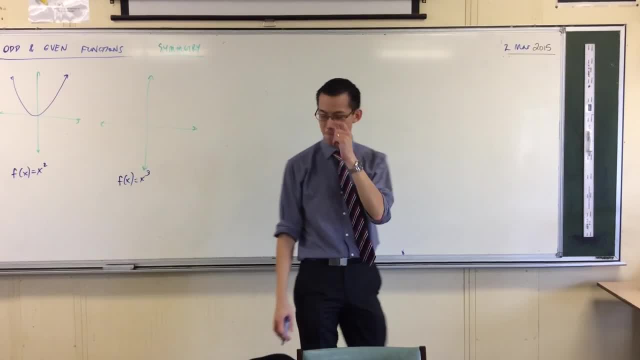 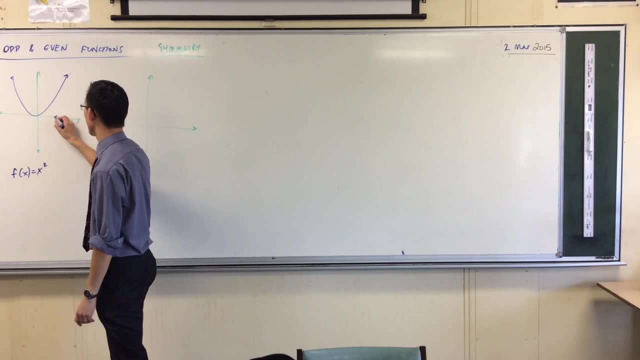 This is also a function of x. I could call them different things, but it doesn't matter. okay, Now you can see that this is a function of x. This thing is symmetrical, right? So, for instance, if I took a value like, x equals 2,. 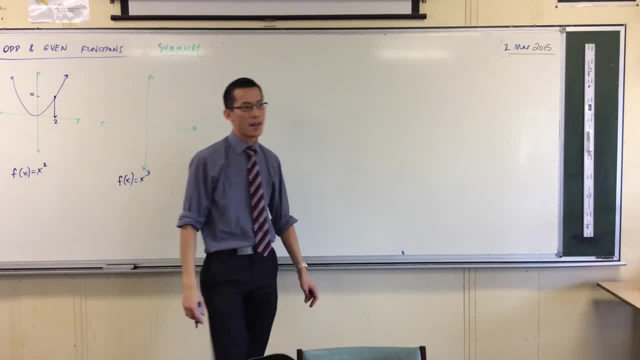 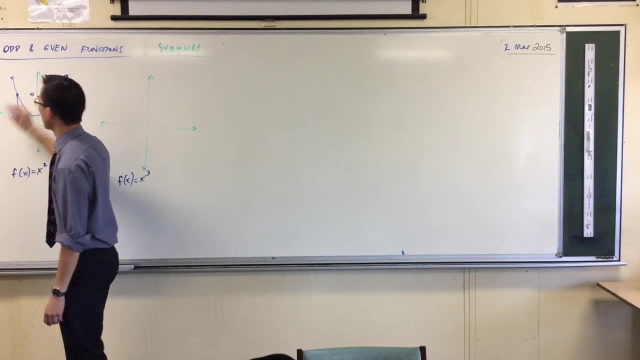 and I draw that up to a certain value, you'd get 4, right. And if I go to the opposite side of the y-axis and I go to minus 2, and I draw my point up, I will get the same value, right. 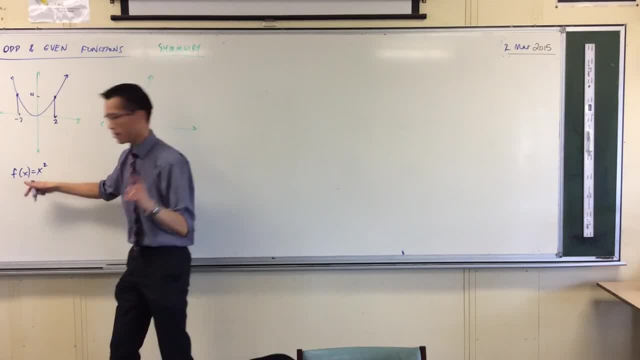 So the way of saying that with this language is to say that f of 2, right, My x value is 2, so that's why it appears where the x is. It's equal to f of minus 2, okay. 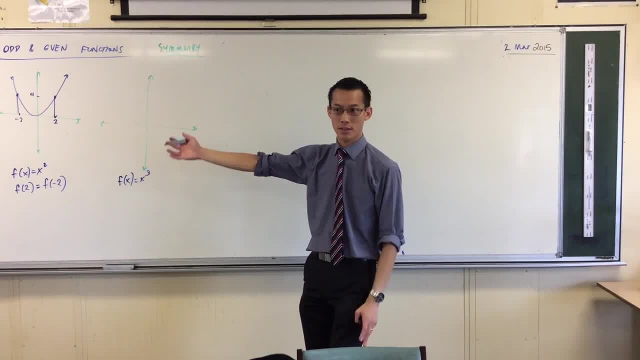 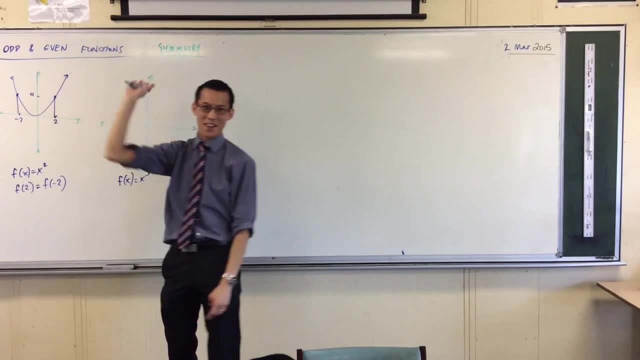 And actually I can take this for any value of x on this particular function, because it's symmetrical all the way. It's not like it gets to you know a million and five and then decides, look stuff, that I don't want to be symmetrical anymore. 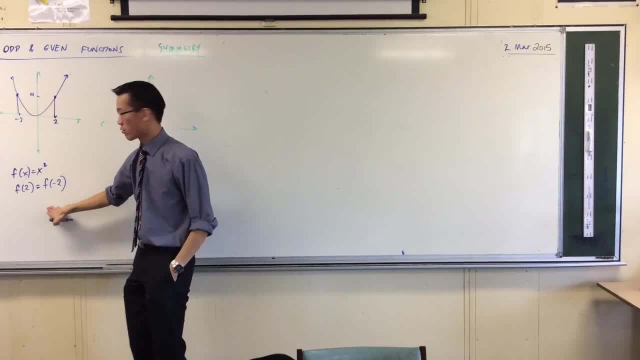 All values of x. right, It's going to do that. So I can state this generally. I don't just have to put particular values. I can say: f of x equals f of minus x for any value of x Right. 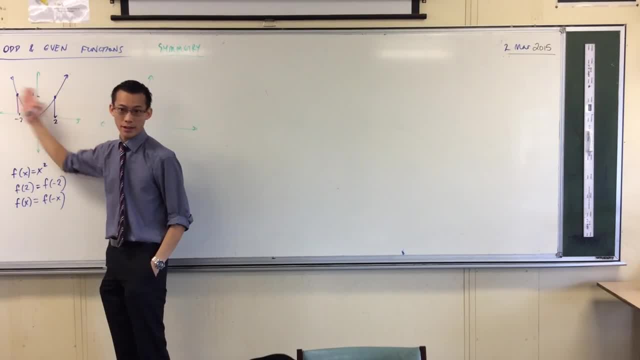 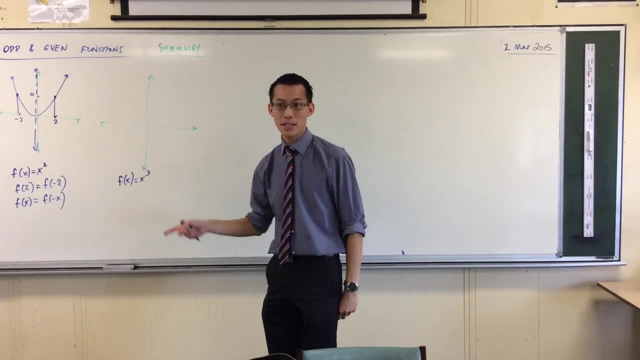 That's what gives this. so we call: well, this is reflectional symmetry, isn't it? It's symmetrical about the y-axis, okay, And we call this even symmetry. In a second I'll ask you why. Let's come over to this guy, right. 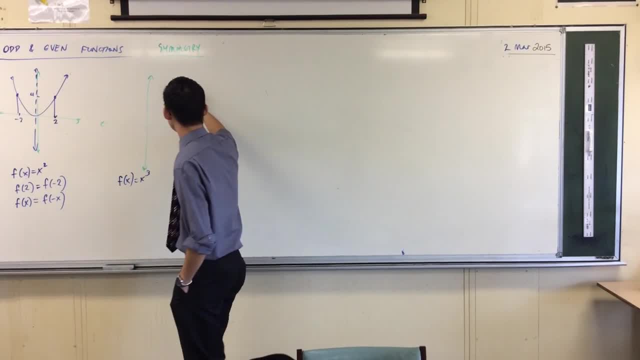 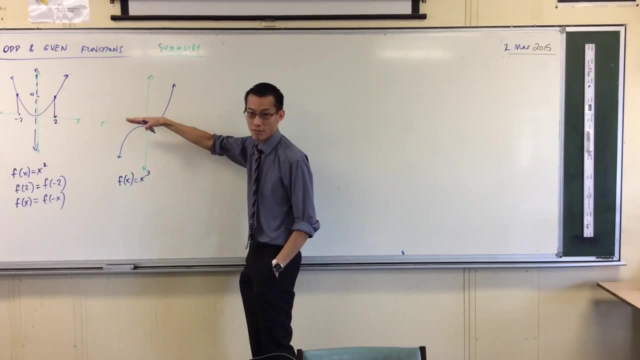 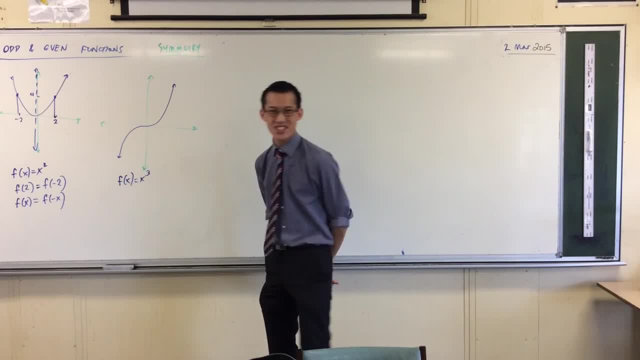 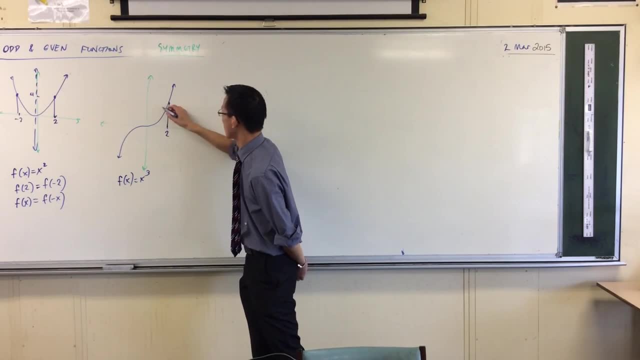 Now, there's still symmetry here. There's still symmetry here, But it's not the same kind. Okay, For instance, I take the same value, 2.. Okay, And you go up to the corresponding value up here, Right. 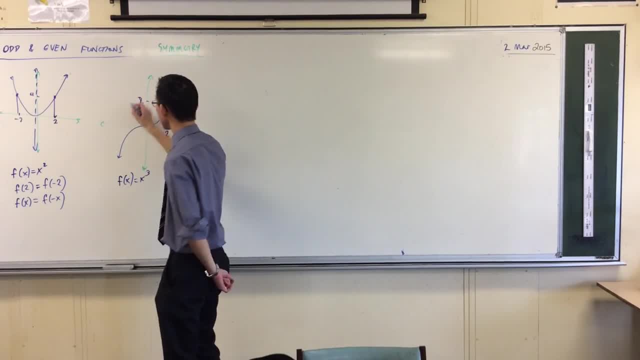 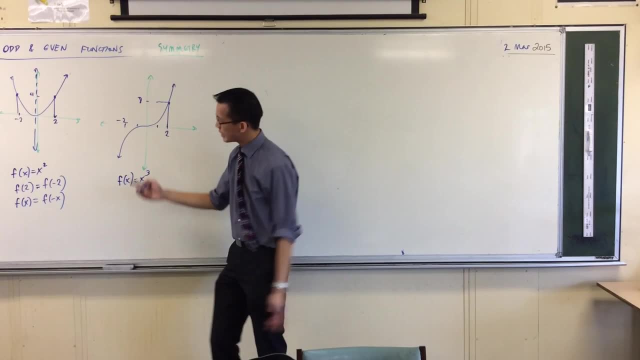 It's going to be 2 cubed, which is 8. 8. Now, when I take the same value on the other side and I go to minus 1,, minus 2.. Okay Well, unlike here, I'm not going up to the same value, 8.. 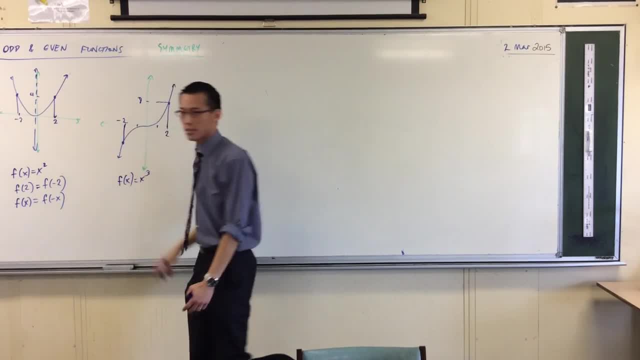 Clearly Right. But what I am going to is the same value but negative right, Because minus 2, all cubed of course, is minus 8.. Okay, so how would I say this? Look at that statement we made over on the left right. 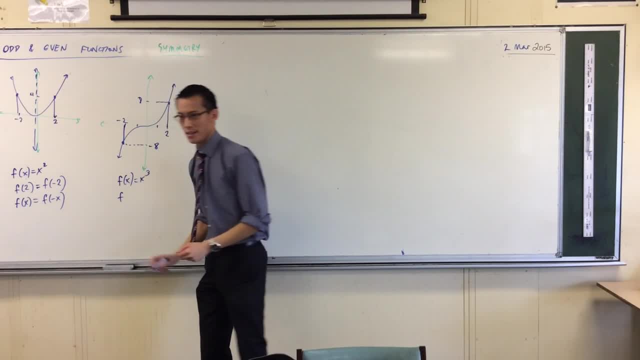 Yeah, go ahead. f of negative x is equal to negative f of 2.. Okay, I'm going to come to that in a second. I just want a statement from these numbers, right, f of 2 is 8.. We'll get to the generalization in a second. 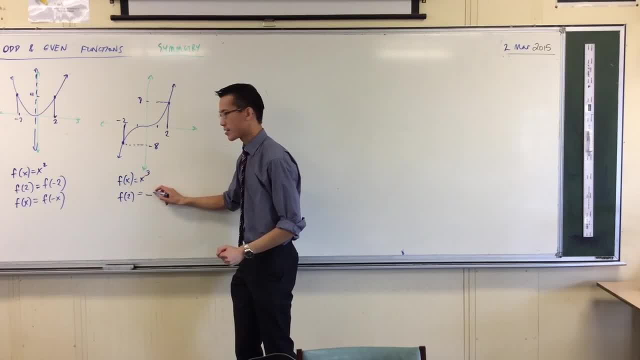 And that's equal to minus f of minus 2.. Okay now, excuse me, You can see this minus sign. I could kick him over here if I wanted. I can multiply both sides by minus 1.. It's the same statement like so okay. 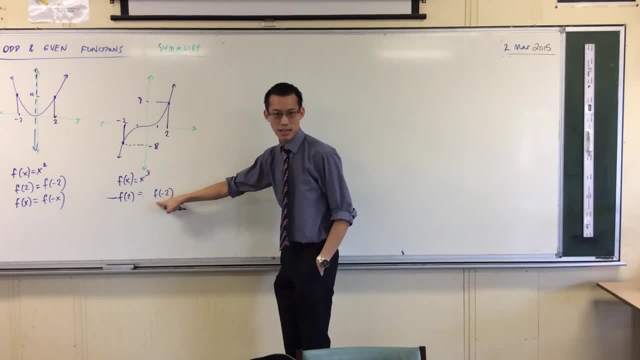 Because f of 2 is 8, so this would be minus 8, which is, of course, the same as f of minus 2, minus 8.. So now, if I state this generally, I generally do it the other way around. 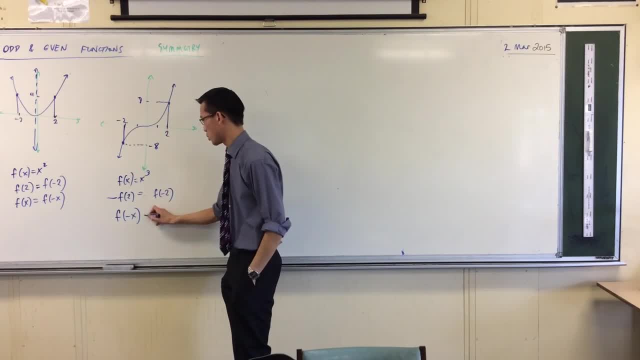 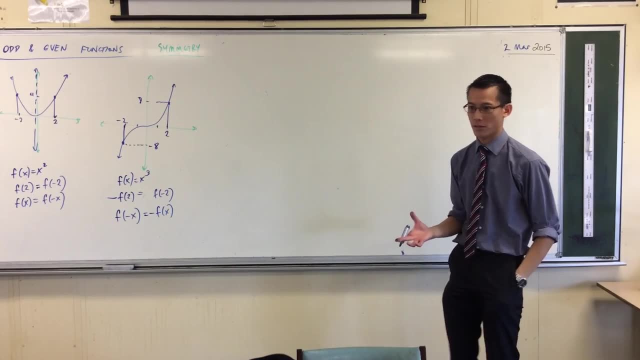 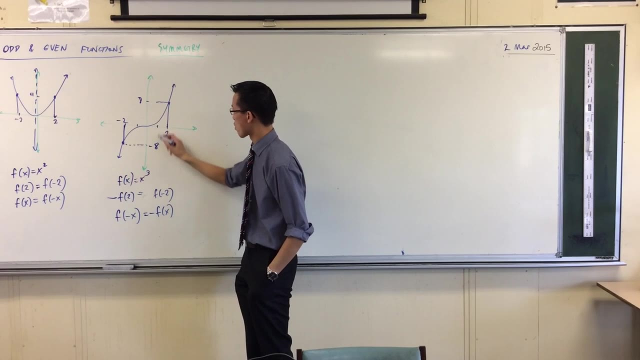 I would say f of minus x is equal to minus f of x, okay, So what I've got here is not reflectional symmetry, right? It's not reflecting across there, It's not even reflecting across here, okay. In fact, what I've got is rotational symmetry around the origin. 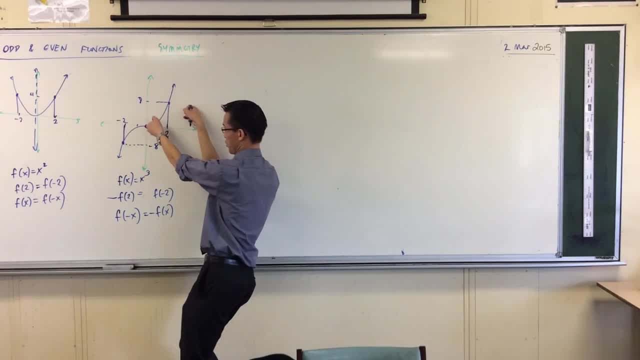 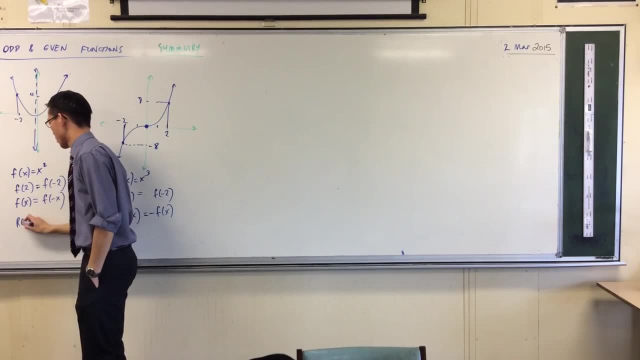 Can you see that If I were to take this part up here in the first quadrant and then just turn it around, you'd get this down here in the third quadrant, okay, So here, reflectional, Okay, and we call that even symmetry or it's an even function. 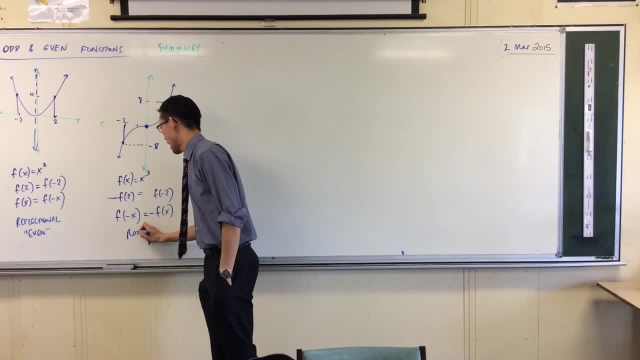 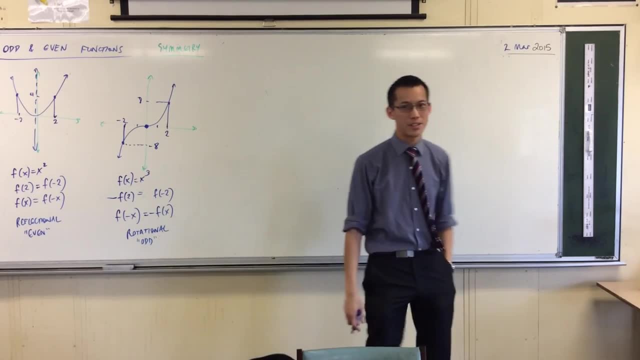 And over here we have rotational symmetry and we call that odd. Okay, now, there are a variety of reasons why they are called odd and even symmetry. But I said I would ask you a second ago why you think they're called odd and even. 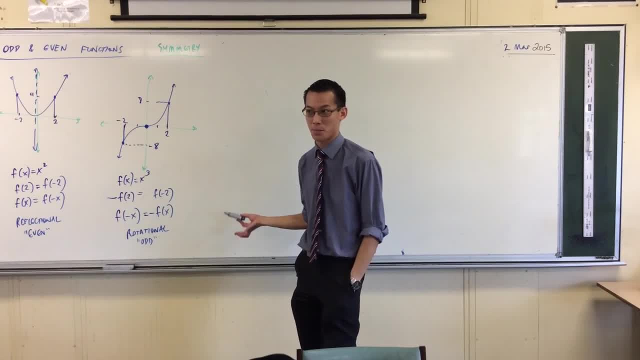 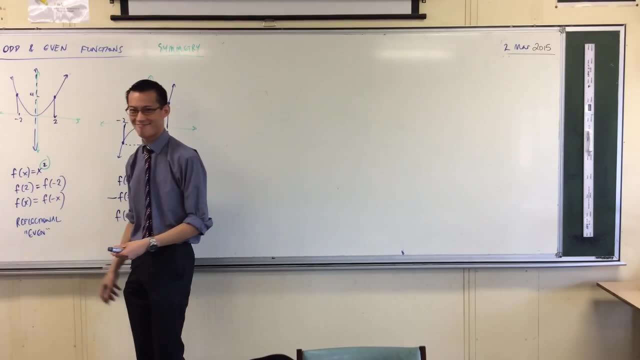 There's one reason which just jumps out at you which I've picked these two examples specifically for this. Yeah, To use an even number. Okay, So you're like even odd. Now, ordinarily I would frown on thinking: oh look, I found one example and another.